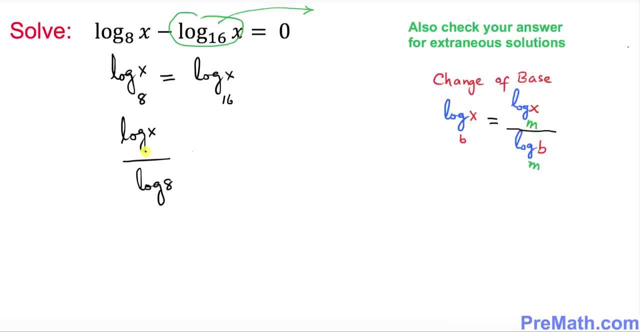 And by default the base is 10, because this is a common log And on this right hand side we have a set of pixels. So if we move these pixels, it's going to be the same as before. So this is a common log. 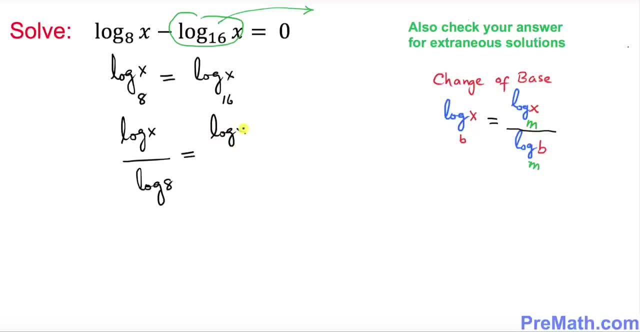 And on this right hand side, we're going to take care of this problem. So we're going to take care of this problem right now. inside, I'm going to do the same thing. log of X divided by log of 16. now the next step. I want you to just look at this: 8 and 16. 8 could be written as 2. 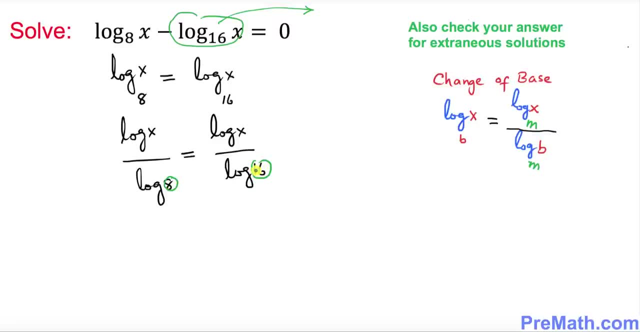 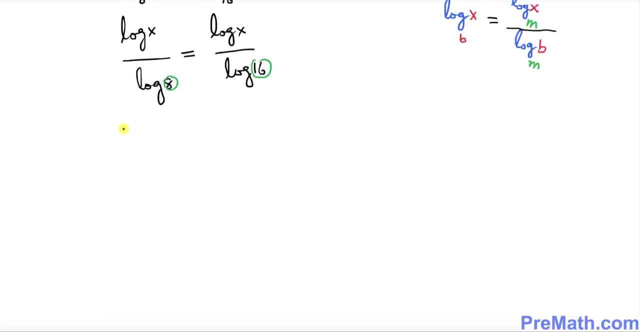 power 3 and 16 could be written as 2 power 4. that's what we're going to do next, so I can write log of X on the top divided by this is I can write log of 2 power 3 equals to log of X divided by log of 2 power 4. now the next we're 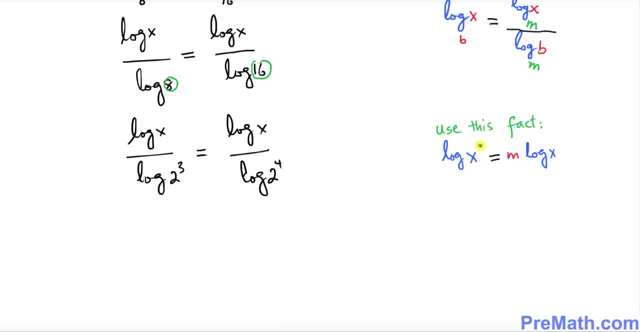 going to be using this fact. if you have a log of X and if you have an exponent power, you can move this exponent to the front. we're going to use the same rule over here on these two exponents. we're going to move this one to the front and I'm going to move this one to the front as. 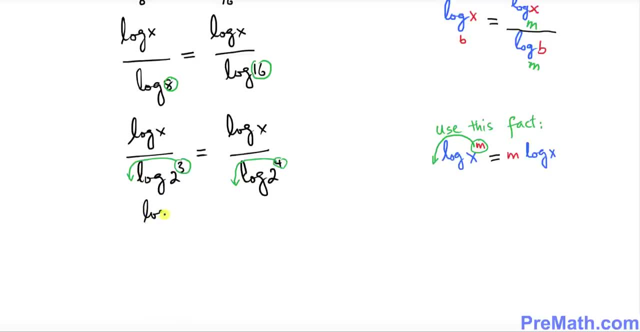 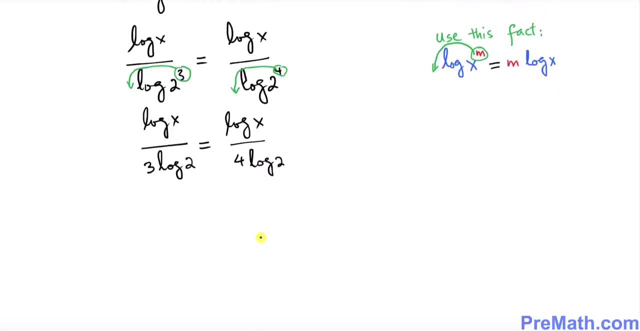 well, so this is going to look like: log of X divided by this. 3 is going to be outside log of 2, equal to log of X divided by 4 times log of 2. so far, so good. now I want you to go ahead and multiply. we want to get rid of this log of 2. I'm going to multiply with: 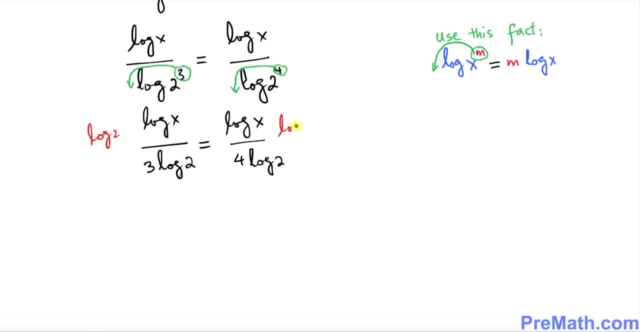 a log of 2 on this side and log of 2 on this side. this log of 2 and log of 2 are gone and this and this is gone. so simply, we ended up with 1 over 3 log of X equals to 1 over 4 log of X. now, as I showed you before, 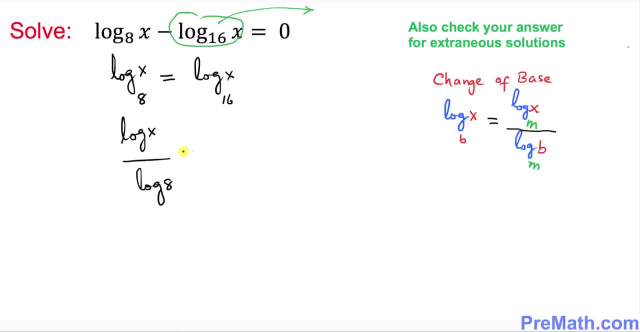 base is 10 because this is a common log And on this right hand side, inside, I'm going to do the same thing: log of X divided by log of 16. now the next step. I want you to just look at this: 8 and 16. 8 could be written as 2. 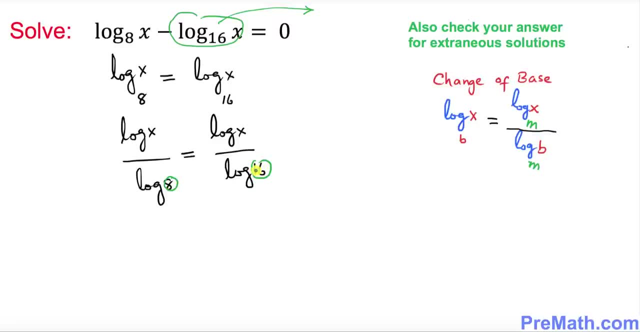 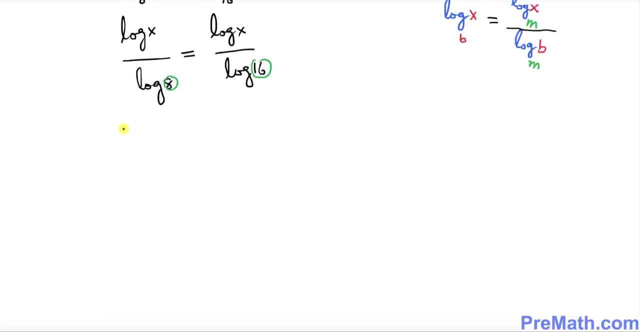 power 3 and 16 could be written as 2 power 4. that's what we're going to do next, so I can write log of X on the top divided by this is I can write log of 2 power 3 equals to log of X divided by log of 2 power 4. now the next we're 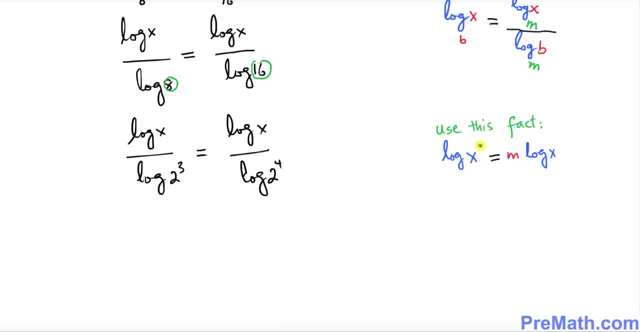 going to be using this fact. if you have a log of X and if you have an exponent power, you can move this exponent to the front. we're going to use the same rule over here on these two exponents. we're going to move this one to the front and I'm going to move this one to the front as. 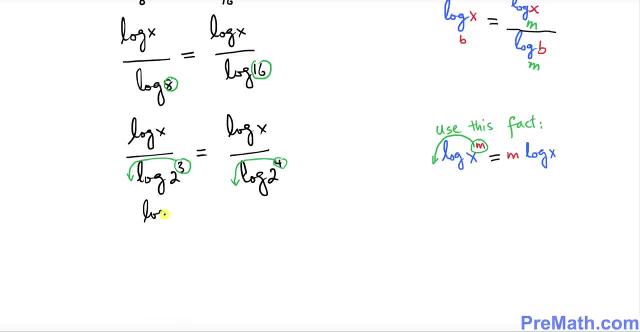 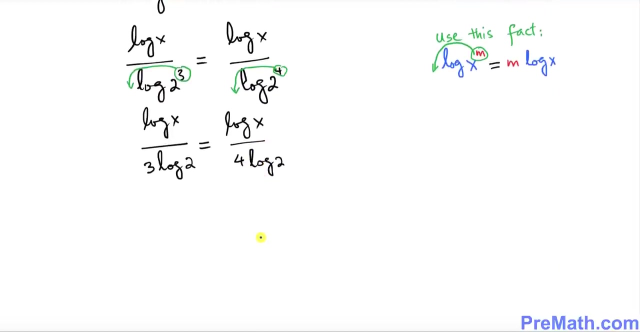 well, so this is going to look like: log of X divided by this. 3 is going to be outside log of 2, equal to log of X divided by 4 times log of 2. so far, so good. now I want you to go ahead and multiply. we want to get rid of this log of 2. I'm going to multiply with: 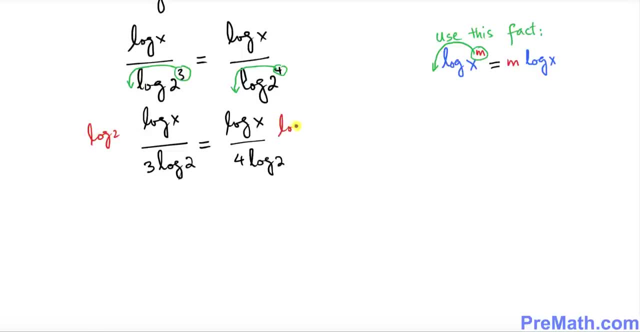 a log of 2 on this side and log of 2 on this side. this log of 2 is going to be 2 and log of 2 are gone and this and this is gone. so simply, we ended up with 1 over 3. log of X equals to 1 over 4 log of X. now, as I showed you before, 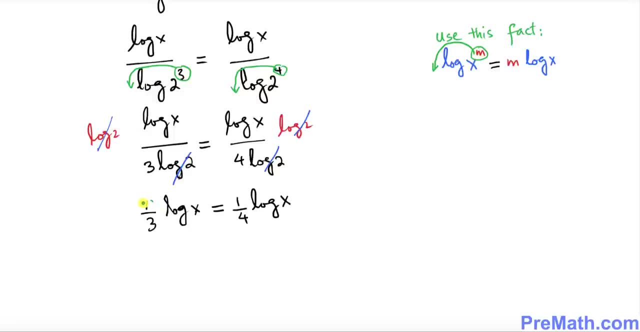 on this one over here. in this fact, this is 1 over 3. if you want to put an exponent, you can put it over here at an exponent, and 1 over 4, I can also put it as an exponent. okay, so this is the way things going to look like I can write. 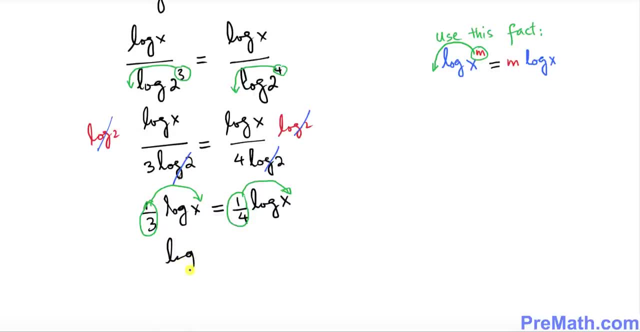 log of X power 1- 1 over 3 equals to log of X power 1 over 4. so now, next, we're going to be applying this fact on this, our given problem. this effect states that if you have a log of X equal to log of Y, then you can just simply write X equals to y here. this is. 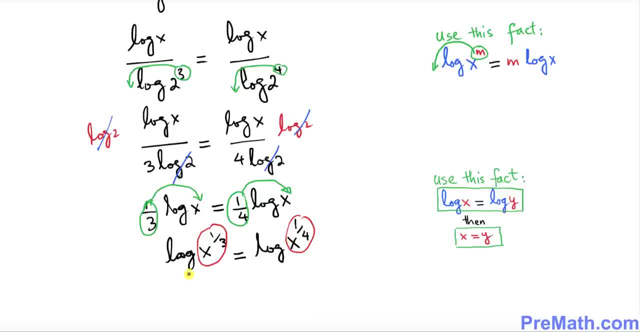 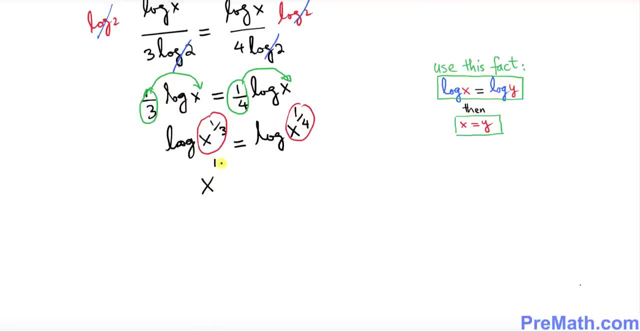 something like X and this is our Y, and we can simply write: X power 1 over 3 equals to X power 1 over 4. right now we have these kind of fractions, the, as exponents. we want to remove these fractions. look at this thing at the. 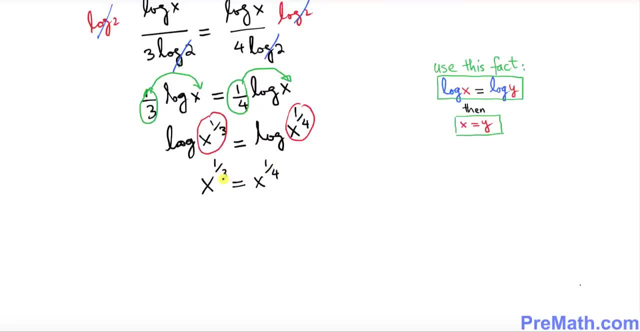 bottom we have a fraction. bottom part is 3 & 4. what is the least common denominator of 3 & 4 is 12. so I'm going to take power 12 on this side and I'm going to take power 12 on this side. so at least we're going to remove those. 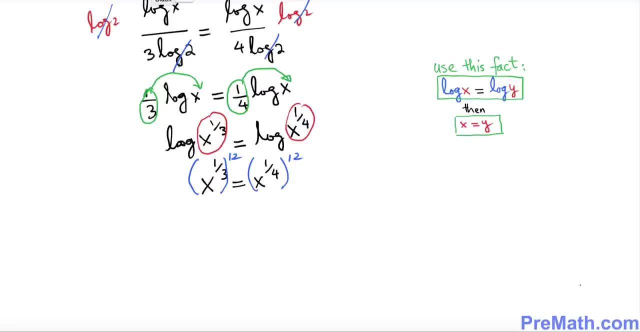 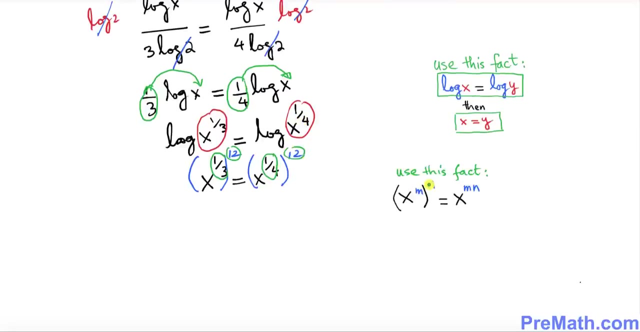 fractions. so simply we're going to be so we have then what 2 exponent: 1, 3rd and 12, 1, 4th and 12. now we will use this fact: if we have X power, M, and then we have another exponent, n, then these two exponents they get multiplied out. so 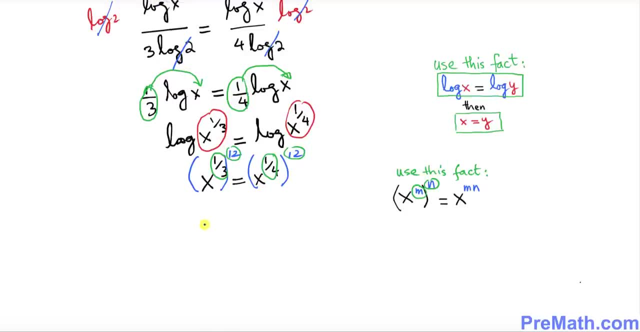 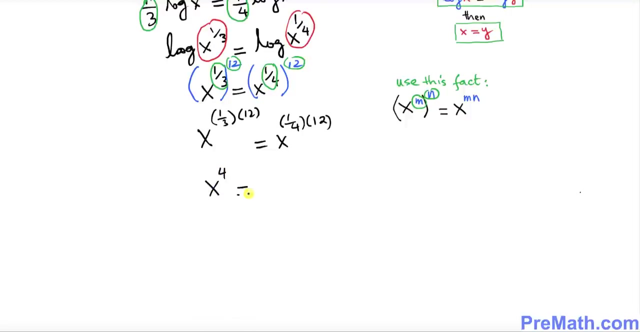 this is the same thing we're going to do over here as well, so I can write X power 1 over 3 times 12 equal to X power 1 over 4 times 12. so far, so good. so this 1 over 3 times 12 makes X power 4 equal to 1 over. 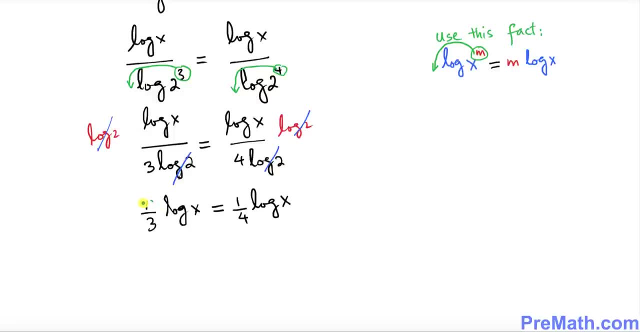 on this one over here. in this fact, this is 1 over 3. if you want to put an exponent, you can put it over here as an exponent, and 1 over 4, I can also put it as an exponent. okay, so this is the way things going to look like I can write. 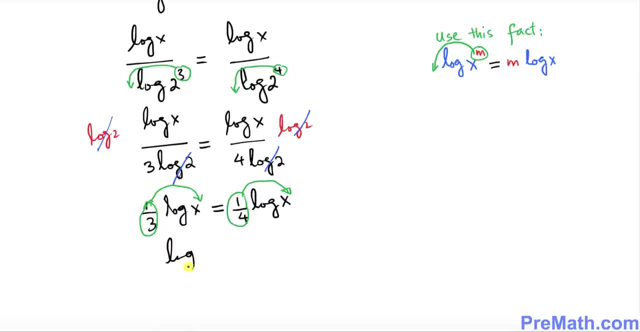 log of X power 1, 1 over 4, 1 over 3 equals to log of x power 1 over 4.. So now, next, we're going to be applying this effect on this, our given problem. This effect states that if you have a log of x equal to log of y. 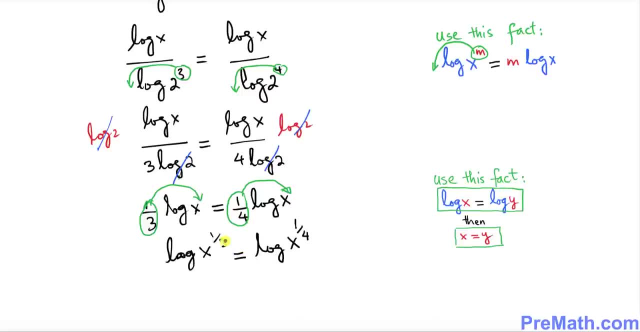 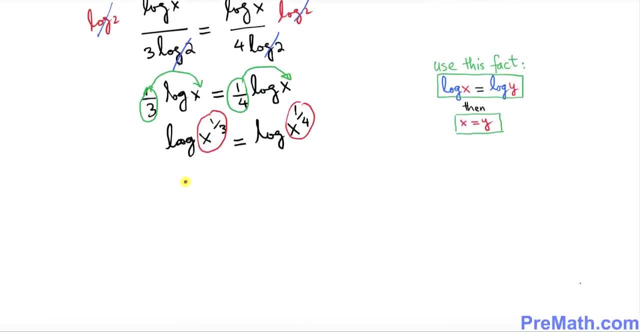 Then you can just simply write x equals to y Here this is our something like x and this is our y, And we can simply write: x power 1 over 3 equals to x power 1 over 4.. Right now, we have these kind of fractions as exponents. 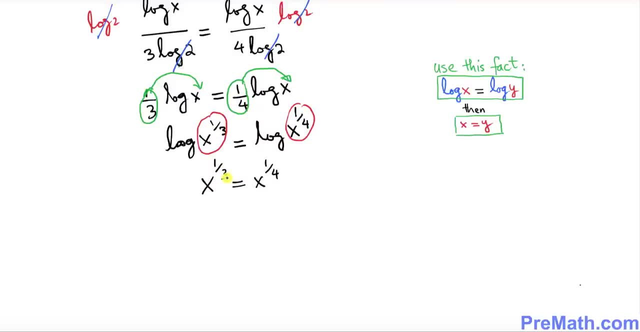 We want to remove these fractions. Look at this thing: At the bottom we have Our fraction. bottom part is 3 and 4.. What is the least common denominator of 3 and 4 is 12.. So I'm going to take power 12 on this side. 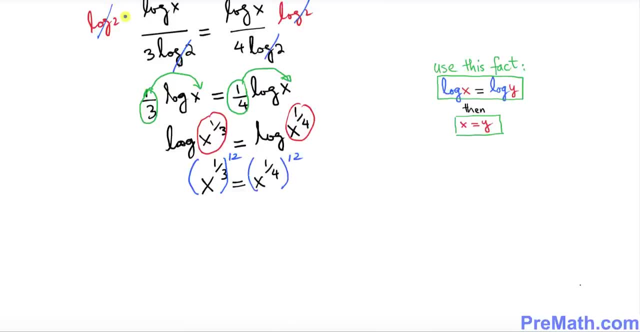 And I'm going to take power 12 on this side. So at least we're going to remove those fractions. So simply, We're going to be. So we have then what? Two exponents: 1 third and 12.. 1 fourth. 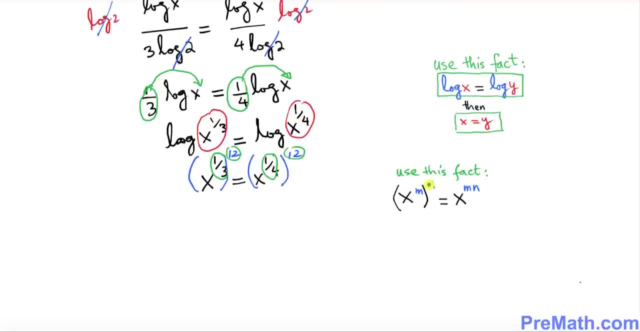 And 12.. Now we will use this fact: If we have x, power m, and then we have another exponent, n, Then these two exponents, they get multiplied out. So this is the same thing we're going to do over here as well. 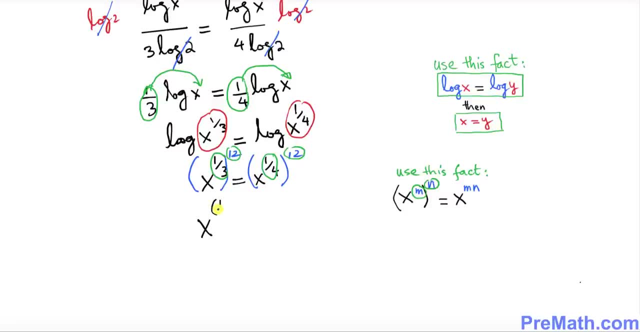 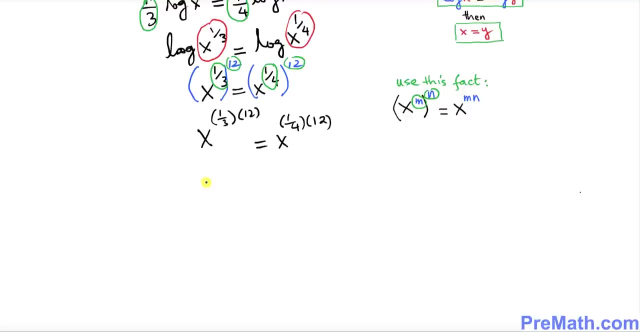 So I can write x power 1 over 3 times 12 equal to x power 1 over 4 times 12.. So far so good. So this 1 over 3 times 12 makes x power 4 equal to 1 over 4 times 12. makes x power 3.. 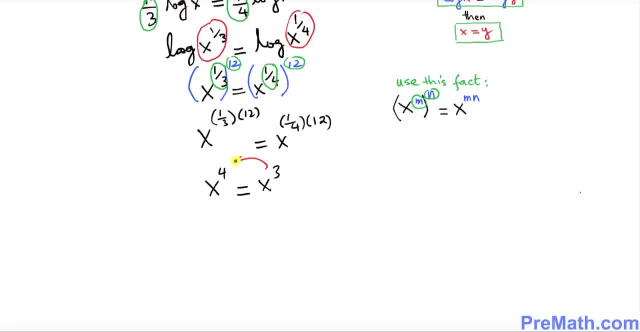 Now I want you to move this x power 3 on the left hand side, So this becomes simply x power 4.. When you move it to the left hand side becomes negative. x power 3 equals to 0.. Now the next thing, what we want to do is: we can. what is the fraction, what is the factored part is going to be? what is in common over here? x power 3 is in common, so I can factor it out. 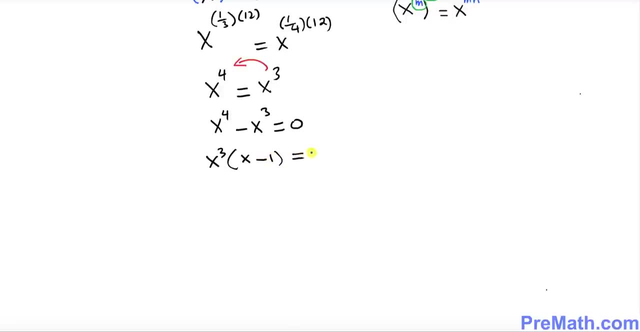 So we got x minus 1 equal to 0. So now I can simply split them up. I can say x power 3 equal to 0 or x minus 1 equal to 0 is if x power 3 is 0, that means x is going to be 0, repeating 3 times, but it's going to be x equal to 0. on this side, x equal to 1 is another solution. 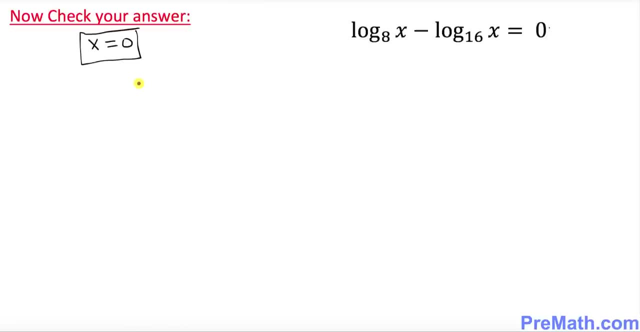 And now we want to check our answer for any extraneous issues. First we check x equal to 0. that means, wherever you see x, replace x by 0. And here I Replaced x by 0 and this is what I got. 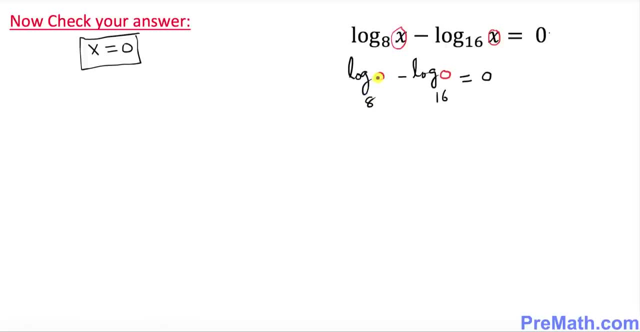 Now look at this thing: we got log of 0 and one thing: you know that the log of 0 is undefined. So that means this whole statement is false. So that means that x equal to 0 is extraneous, So that, in other words, x equal to 0 is not a solution. 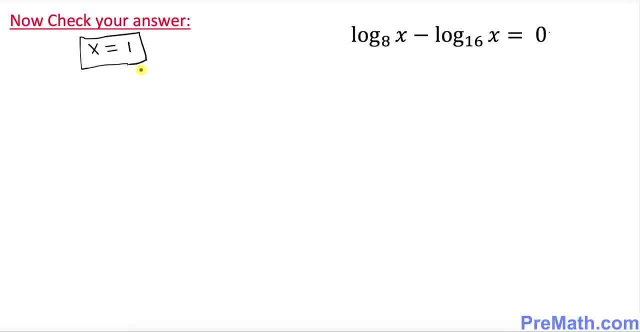 And finally, we want to check our Other solution: x equal to 1 for any extraneous issues. That means, wherever you see x, replace it by 1.. And here I replaced x by 1. right up here, However, log of 1 is always 0, as I put it down. 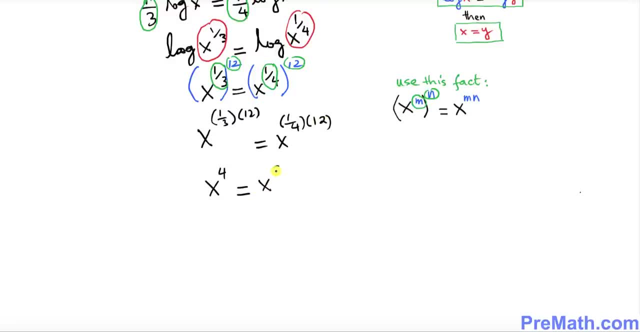 4 times 12 makes X power 3. now I want you to move this X power 3 on the left hand side, so this becomes simply X power 4. when you move it to the left hand side becomes negative. X power 3 equals to: 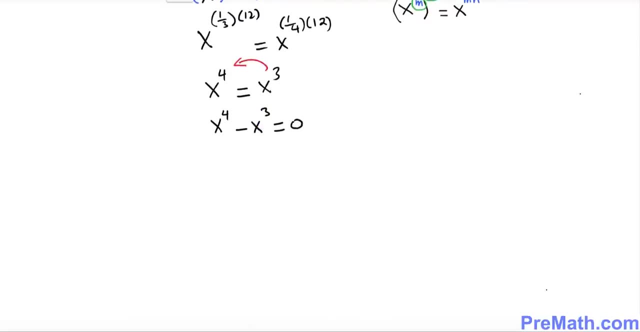 0,. now the next thing. what we want to do is: we can. what is the fraction? what is the factored pod is going to be? what is in common over here? X power 3 is in common, so I can factor it out. so we got X minus 1. 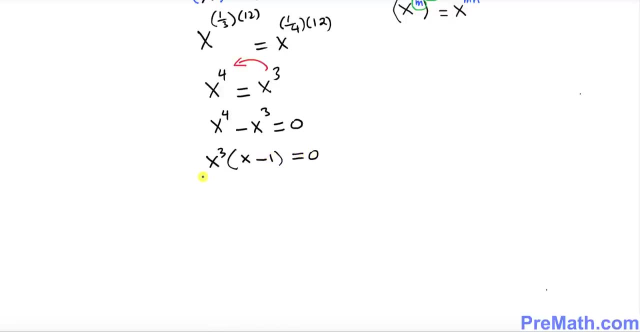 equal to 0. so now I can simply split them up. I can say X power 3 equal to 0, or X minus 1 equal to 0. to 0 is: if X power 3 is 0, that means X is gonna be 0, repeating three times. but 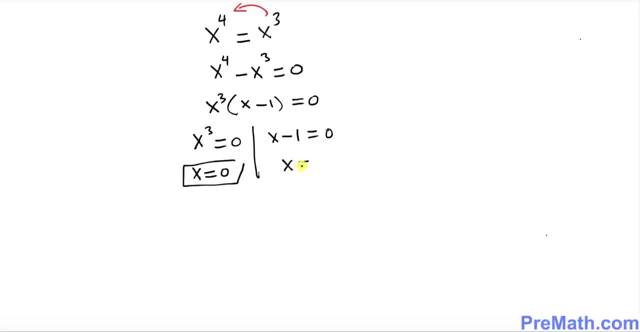 it's gonna be X equal to 0. on this side, X equal to 1 is another solution. and now we want to check our answer for any extraneous issues. first we check X equal to 0. that means, wherever you see X, replace X by 0, and here I replaced X by. 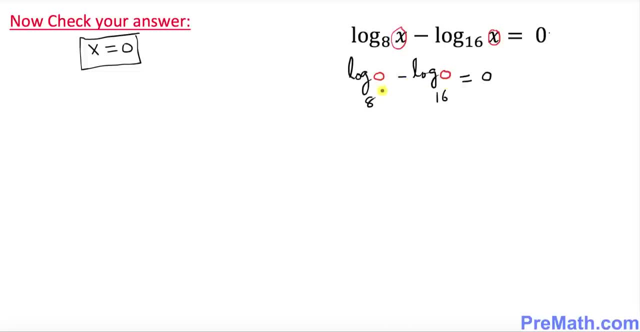 0 and this is our what I got. now look at this thing: we got log of 0 and one thing: you know that the log of 0 is undefined. so that means this whole statement false. so that means that X equal to 0 is extraneous. 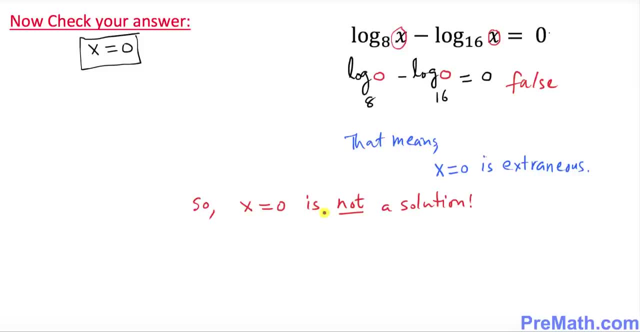 so, in other words, x equal to 0 is not a solution. and finally, we want to check our other solution: x equal to 4, 1 for any extraneous issues. that means, wherever you see X, replace it by 1, and here I replaced X by 1, right up here.